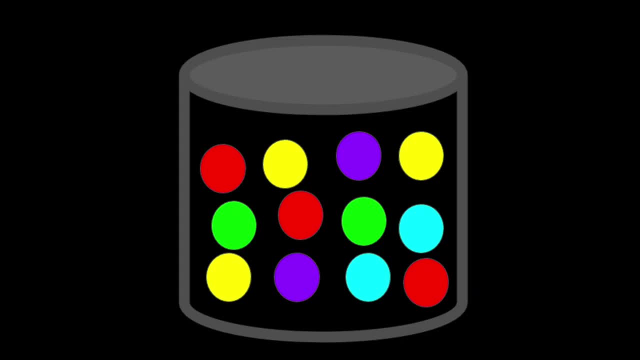 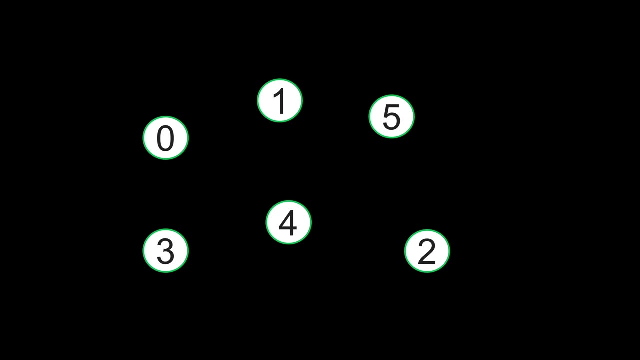 So let's begin by talking about what union find does. Imagine if you had some objects and you want to group them together according to some criteria. So one such grouping might be this. Now, once you have completed the grouping, you would want to know certain properties about the. 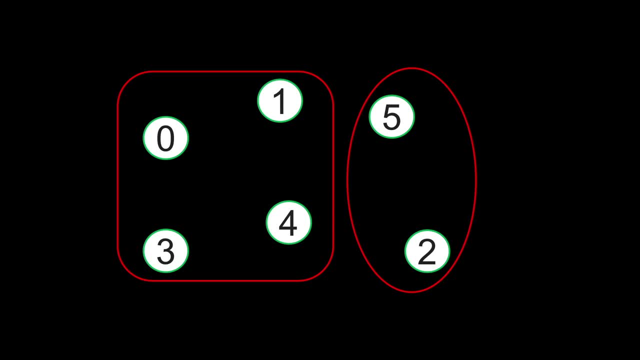 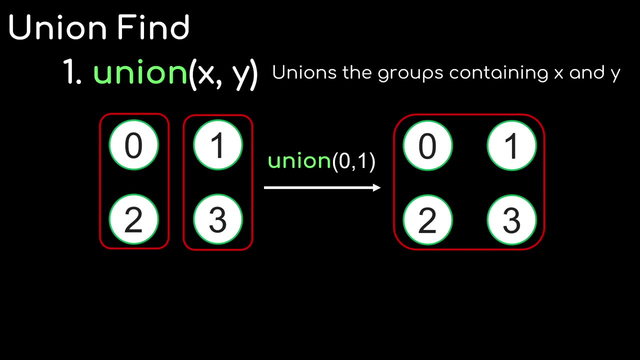 groups, such as how many groups there are and if two objects belong to the same group. The union find data structure, as its name suggests, supports two operations. The first one is called union, which takes as input two elements, x and y, from the set of objects. 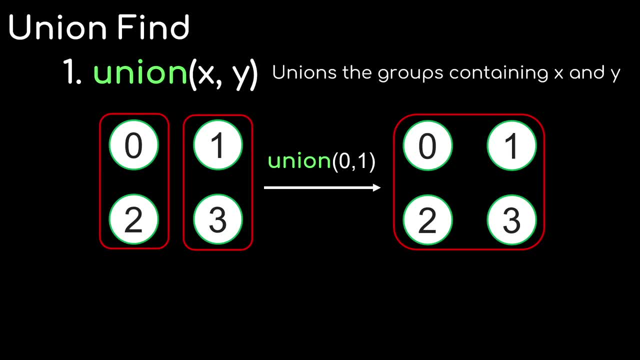 and it joins or unions the groups containing x and y. For example, we can start with 0 and 2 belonging to the same group and 1 and 3 belong to the same group, and when we call this function union 0, 1,, it joins or unions the groups containing 0 and 1.. So the final result would be: 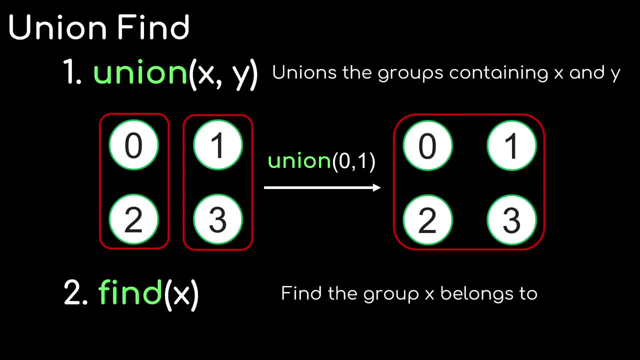 all four objects belonging to the same group. The next one is called union, which takes as input two elements- x and y- from the set of objects, and it joins or unions the groups containing x and y. The final result would be all four objects. 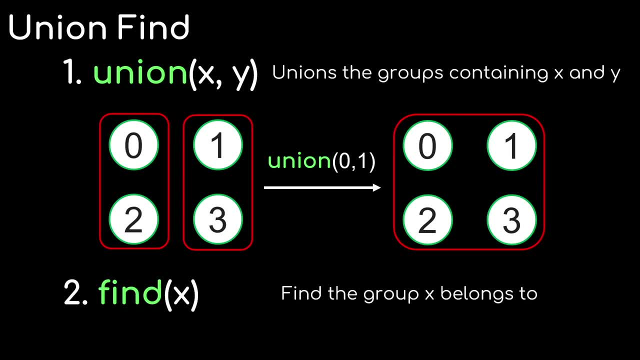 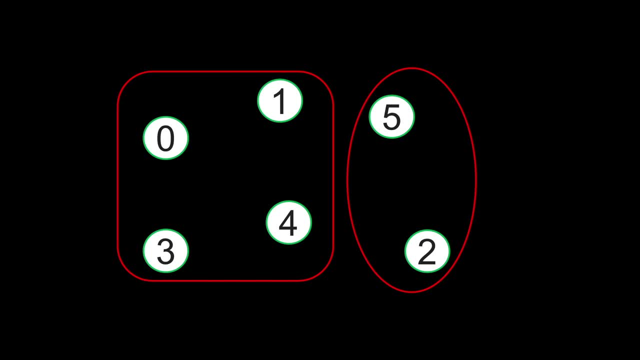 belonging to the same group and 1 and 3 belong to the same group. The next operation is called find, and it takes a single object, x, as the input and returns the group that x belongs to. So now let's see how we can implement union find. We will first walk through the ideas and discuss. 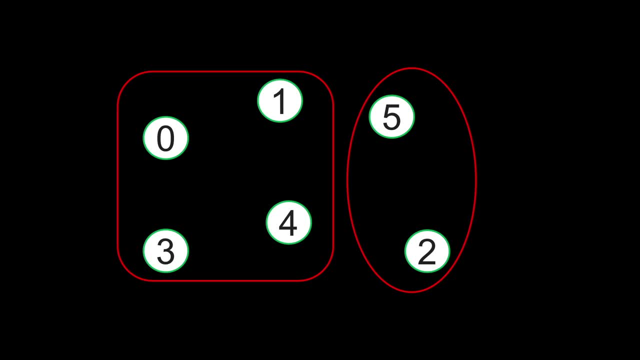 the code at the end. Union find is useful in graph-type problems, so our first step will be to cast the grouping in the form of a graph, And the way we do that is to connect all the objects that belong to the same group with an edge like so: 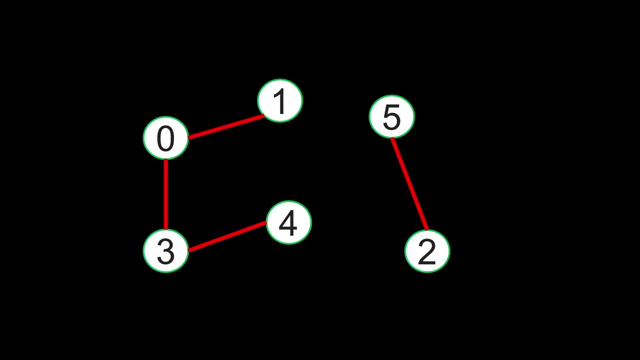 Now remember, we need to find a way to determine which group each element is in. To do so, we designate a representative element for each group. This element will represent the entire group it belongs to, in the sense that the find function will always return the representative. 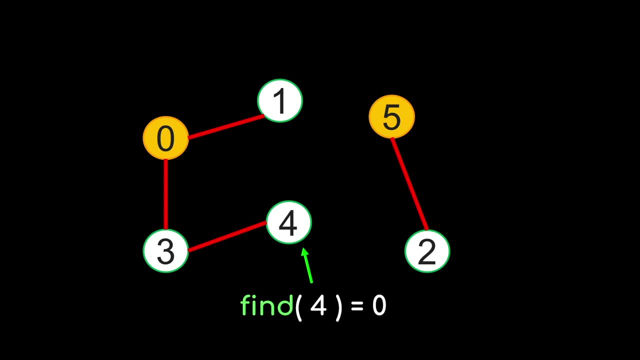 For example, when we call find, the representative of the group that 4 belongs to is 0, so therefore we return 0. And of course the representative will return itself. As another example: when we call find, we return the representative of the group 2 belongs. 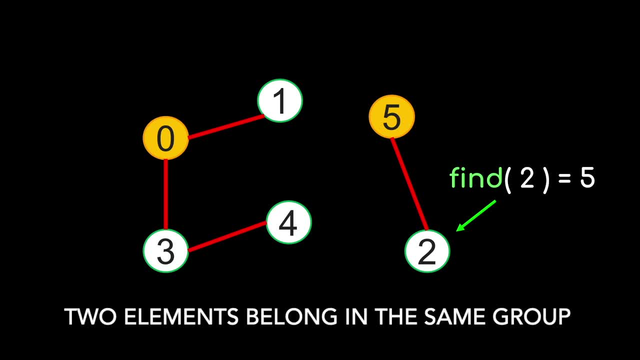 to which is 5.. Notice that two elements belong to the same group if, and only if, they have the same representative. So the representative provides a way of checking if two elements belong to the same group. So now we need to implement the other function, which allows the union of two groups. 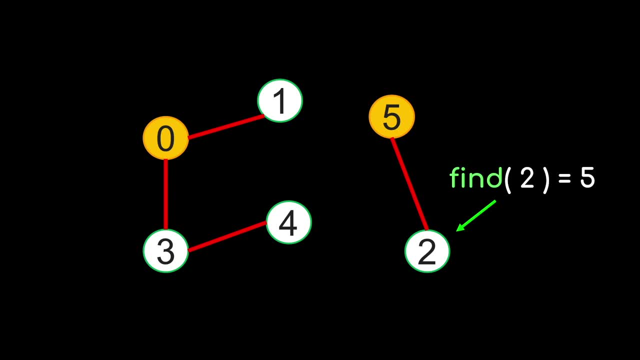 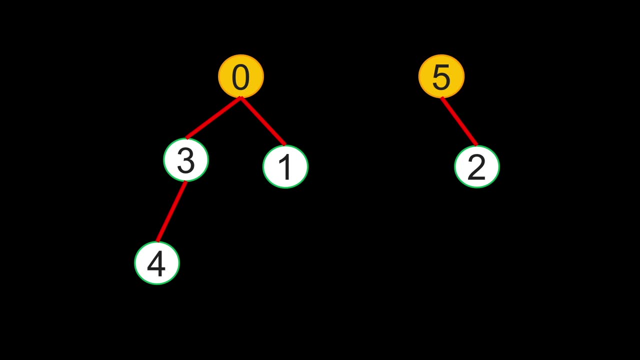 And to do that, let me rearrange this graph in a suggestive way. I've now put the representatives at the top and the rest of the elements of the group towards the bottom. Now each group is represented as a tree, with the root being the representative. 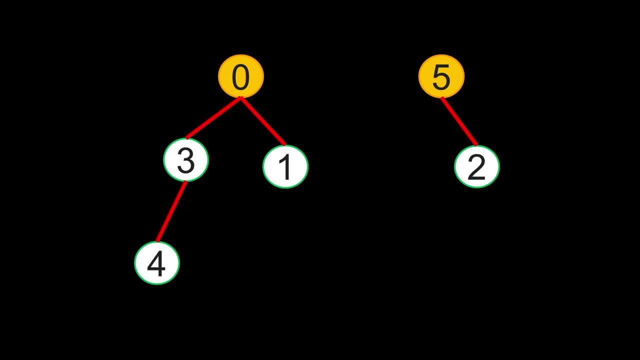 With this, we can introduce the notion of parents and children For any given element. how do we find the representative? Well, we must travel upwards the tree towards the root. In other words, we need to keep traveling towards the parent until we reach the top. 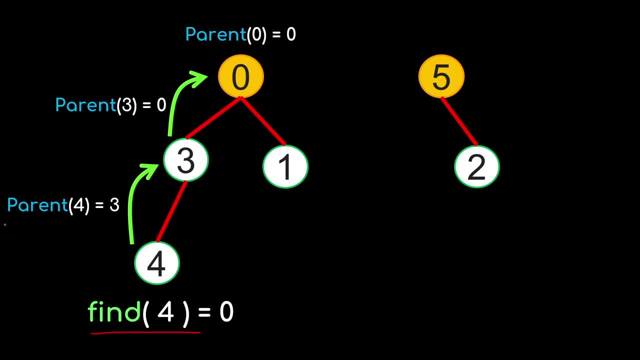 As an example, Suppose we want find The parent of 4 is 3,, so we travel upwards to 3, and the parent of 3 is 0,, so we travel up to 0. And we would know when to stop if we just use the simple convention that the parent 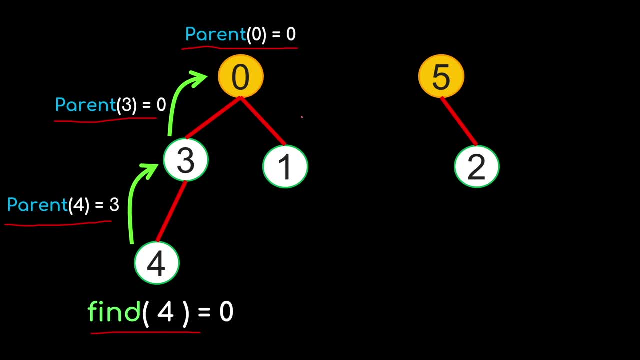 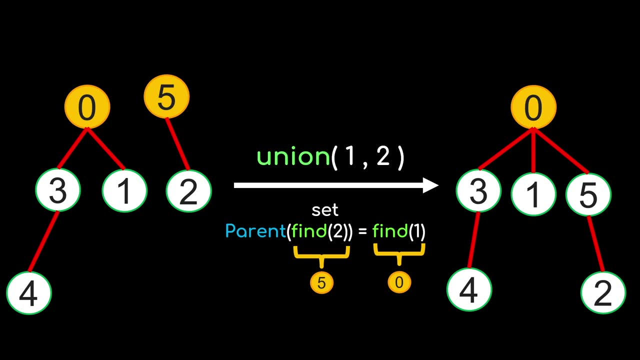 of a root is itself. So if we can keep track of the parent of every object, then we can very easily travel upwards the tree towards the root. So what about the union operation? Well, in this new interpretation, the representatives are the roots of the trees. 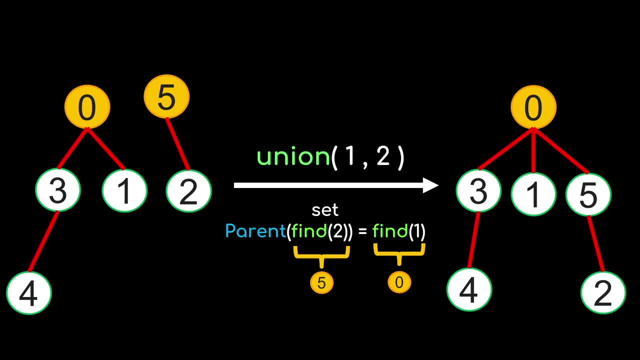 So if we want to union two trees, we can just set the root of one tree to be the child of another. For example, suppose we want to union 1 and 2.. 5 is the root of 2, which we can get by calling find, and similarly 0 is the root. 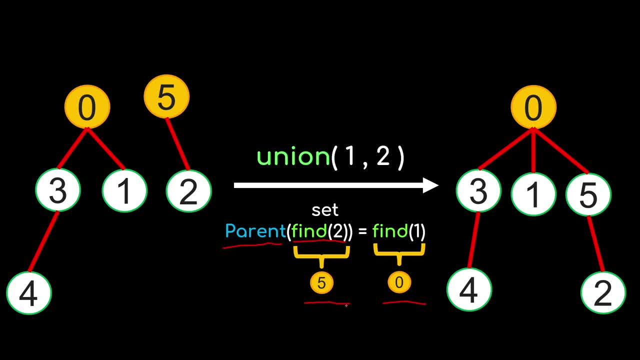 of 1.. We then set the parent of 5 to be 0, and what this does is that it sets 5,, which used to be a root, now as a child, of 0. And all of the elements that used to be in the tree are now the root of 1.. 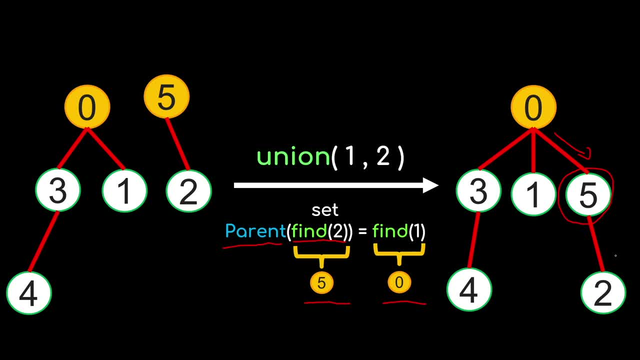 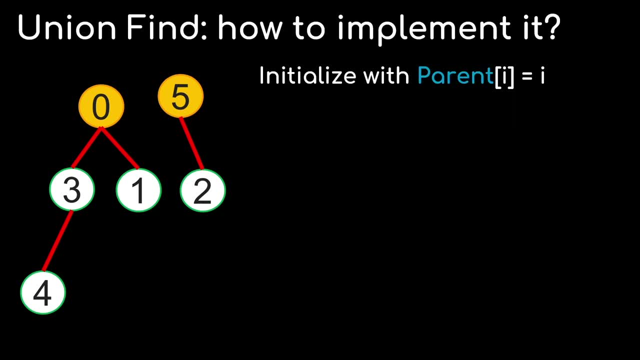 And all of the elements that used to be in the tree rooted at 5 now have a root of 0. And now these two trees have been unioned. Now we have the basic idea. let's discuss how we can implement this in code.